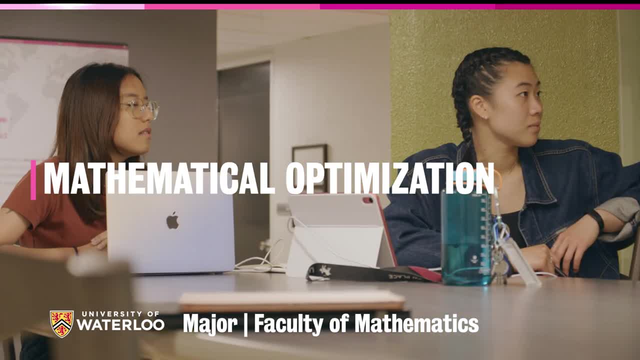 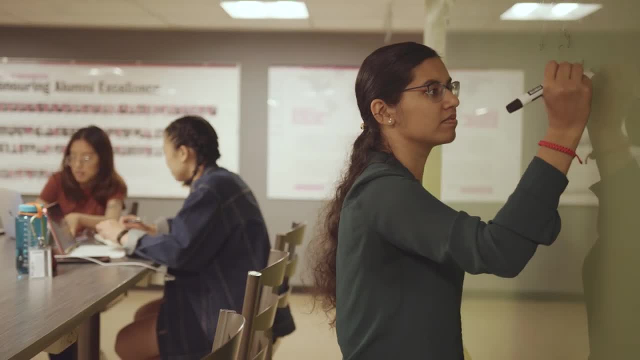 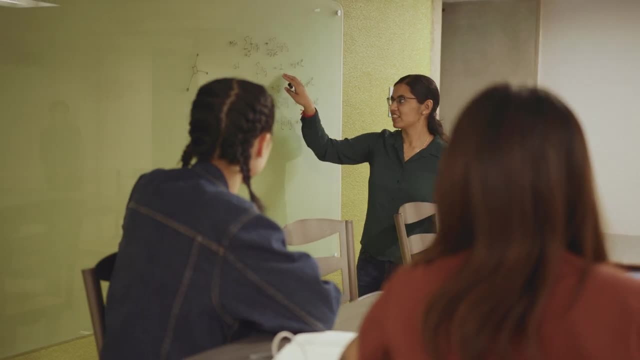 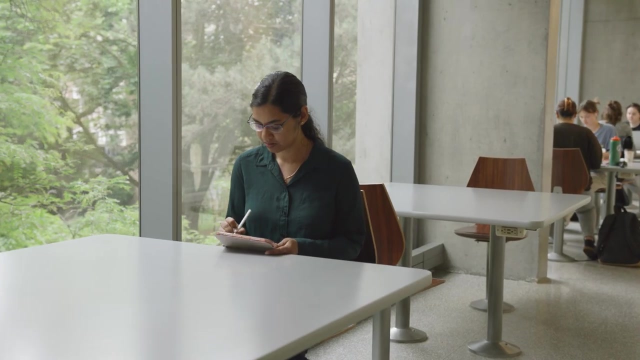 For me, math was always about problem-solving, and two courses that I took in my undergrad- Introduction to Optimization and Computational Discrete Optimization- introduced me to very interesting problems, and I also found the techniques we used to tackle these problems very interesting. Sometimes it felt a bit like magic. Optimization, specifically, is about solving. 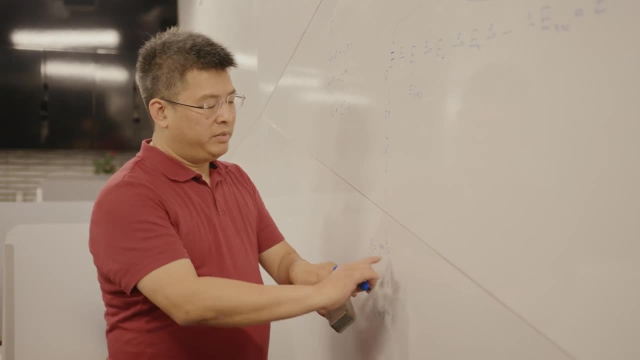 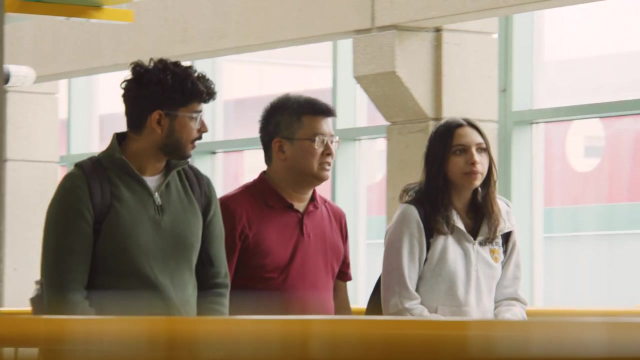 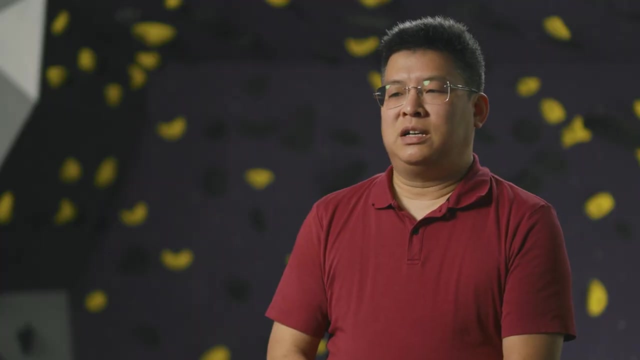 problems where you're trying to optimize some outcome, but as you do this, you've always got these real-world problems in mind. How do I maximize the performance of this financial portfolio? How do I target my political advertising to get the most votes? And so, if you are the kind 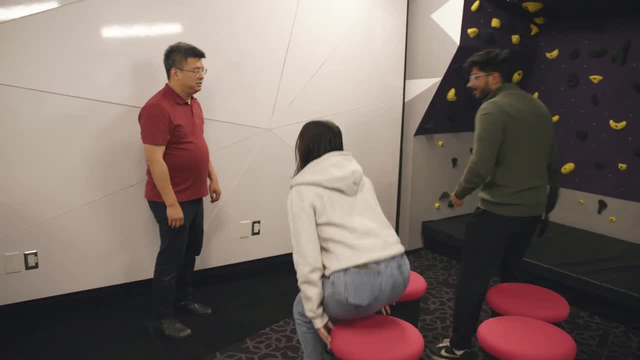 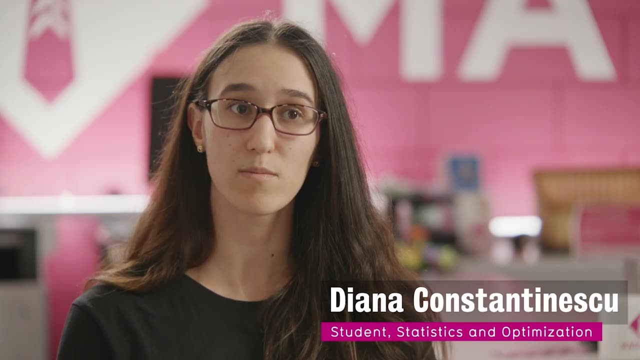 of person who is interested in math for the real-world impact, then you're a good candidate for studying Optimization. Just through the courses themselves, we learn so many algorithms and real-world applications that we can use to solve problems that we don't know how to solve. Just through the courses themselves, we learn so many algorithms and real-world applications that we can use to solve problems that we don't know how to solve. Just through the courses ourselves, we learn so many algorithms and real-world applications that we don't know how to solve. 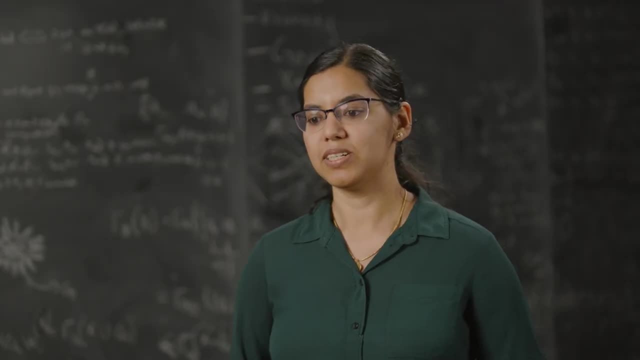 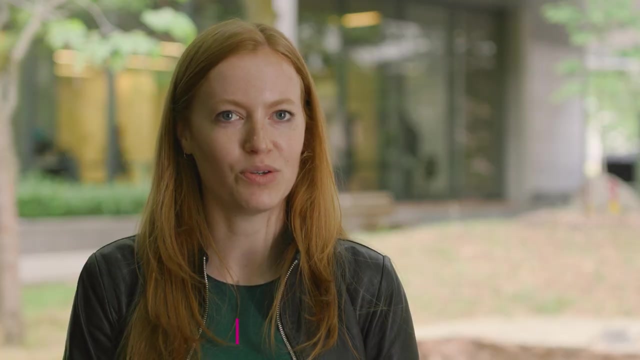 and apply them to those situations. For example, if I'm thinking about transportation, then my constraints often have to do with what routes I'm allowed to take. for instance, You can also go to the finance side, so maybe you want to pick the best portfolio of stocks for some client. 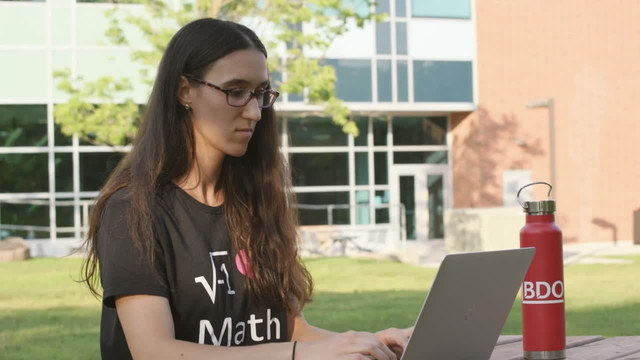 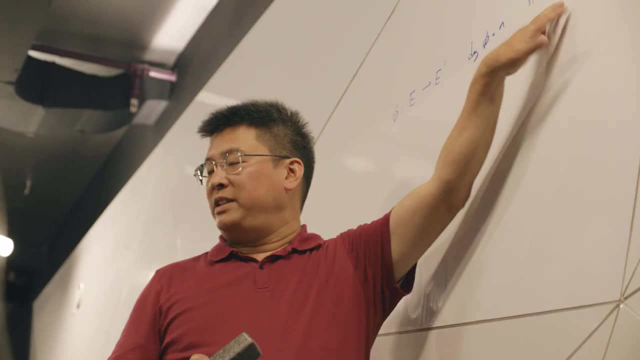 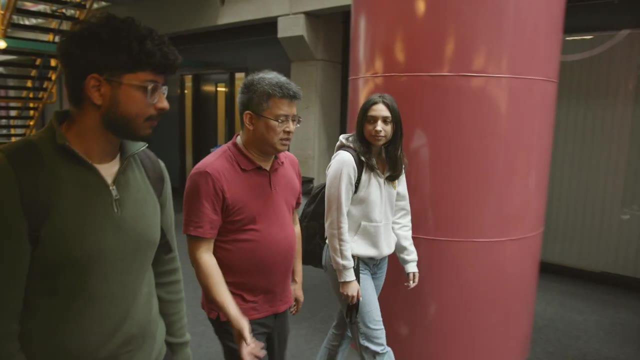 A big one would probably be within supply chain and food manufacturers. you might be working there and helping them optimize how all their products come in. Any sort of delivery service- Amazon, UPS, any company that has to schedule resources, airlines and air airplanes, universities and classrooms. What you make of it is up to you, right, but you'll 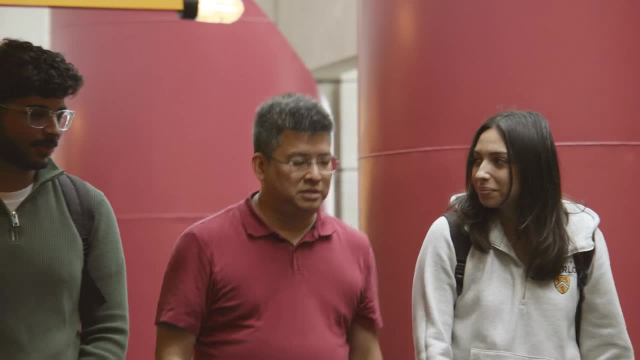 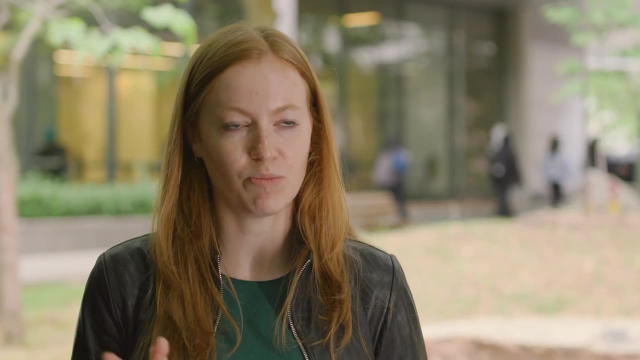 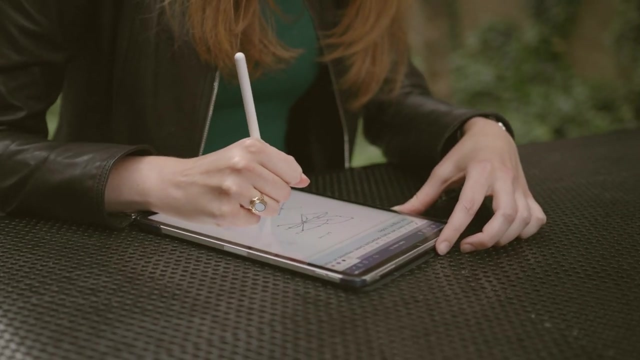 certainly have no shortage of companies or suitors looking for your services. I think the most important thing is just solving problems, and that should excite you. I did an internship at Amazon in Seattle and I realized that if you understand how to solve problems well, you're going to be a good candidate for solving a business's problems. 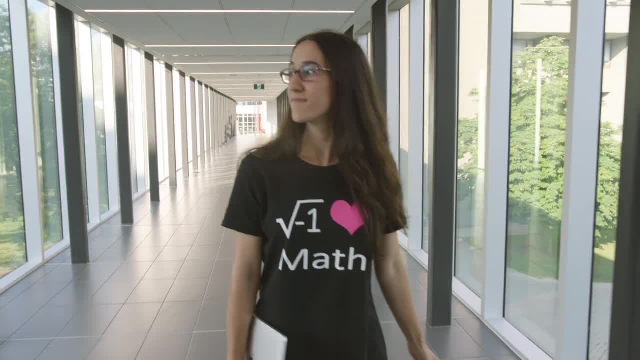 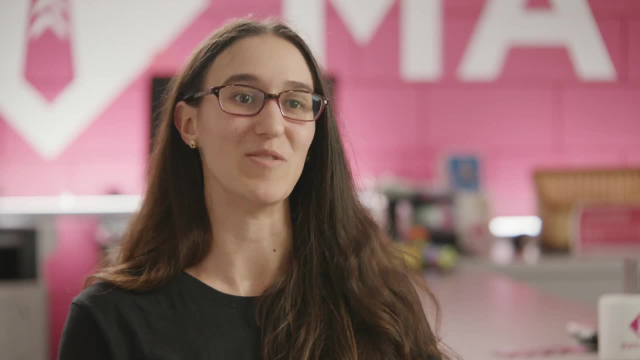 There's so many new things coming out all the time, and so getting that new young perspective and that new view your critical thinking builds so much in this degree and that's the biggest thing you need to succeed in the workplace.